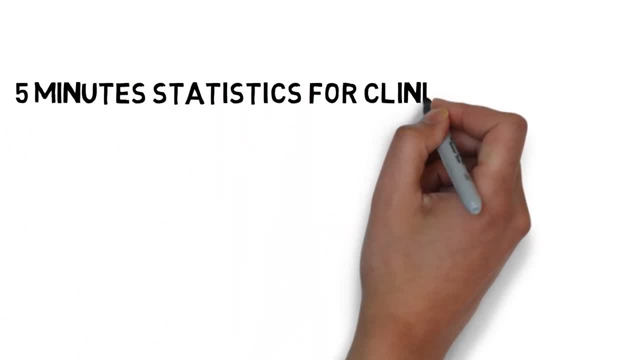 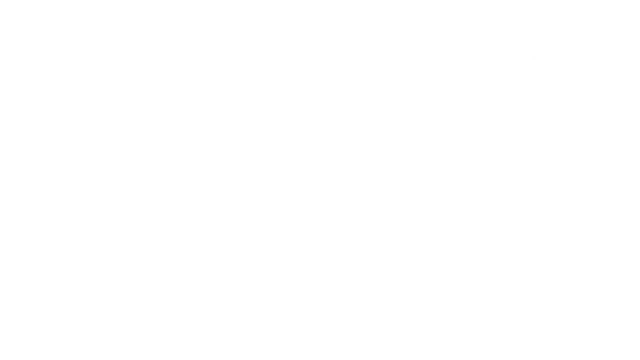 Hi and welcome to 5-Minute Statistics for Clinical Research. My name is Caroline Herwan and I am part of the Biostatistics team at GCP Service International. Conducting a clinical trial is an intricate work with a lot of moving parts. 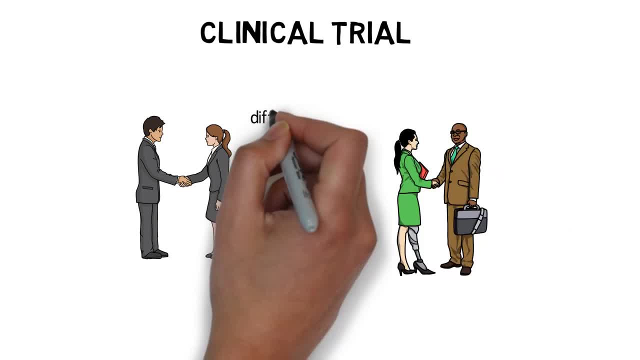 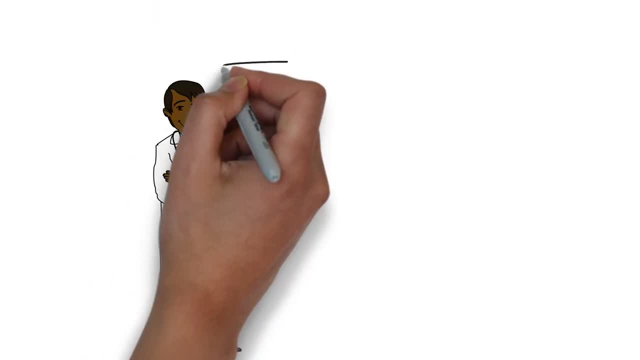 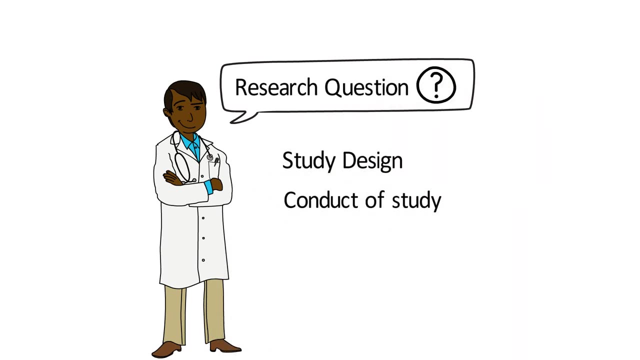 requiring people from many different disciplines to work together smoothly. The aim of every clinical trial is to gain information on a specific research question, though the study design and conduct heavily influences how the data can be interpreted. Therefore, throughout the whole duration of the trial, those working in clinical research 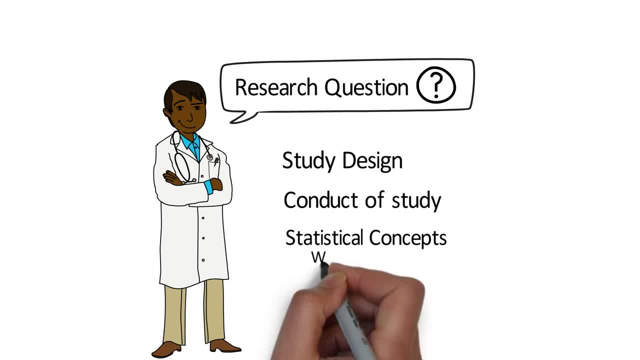 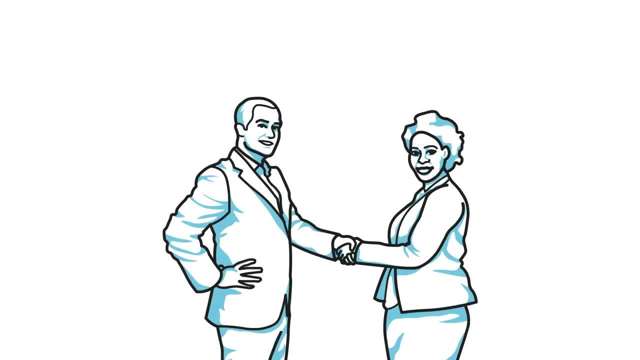 come into contact with statistical concepts that determine what can and what cannot be concluded after the trial. This is, of course, especially the case in the planning phase of each trial and for the interpretation of trial results. Statisticians often have an advisory role in the process of a clinical trial. Therefore, communication should be a key element for 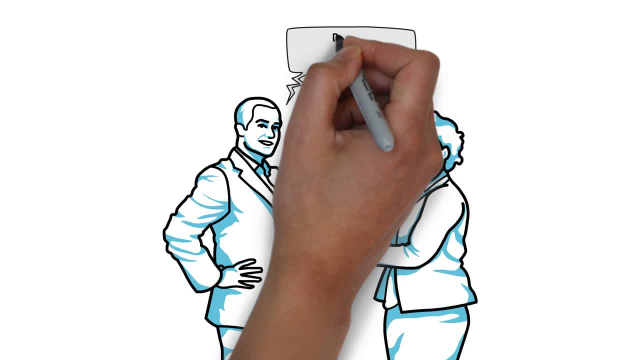 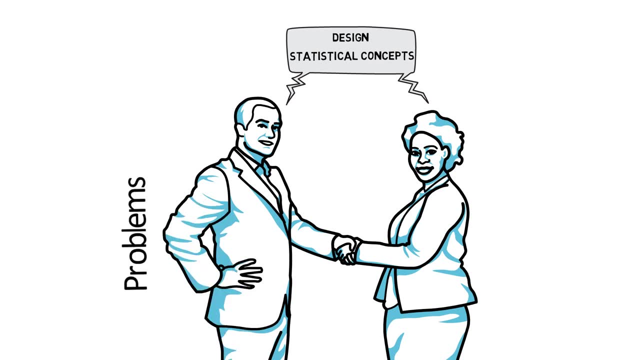 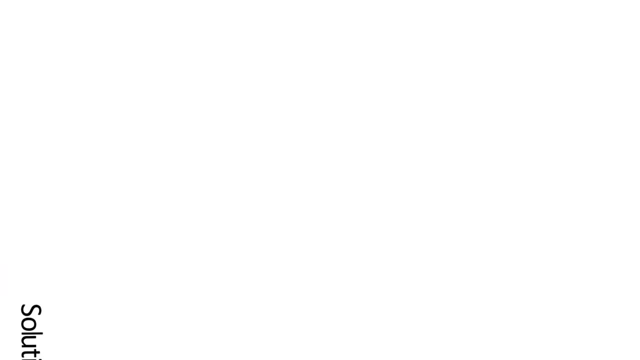 every statistician. The better the important aspects of the design and underlying statistical concepts are understood by the entire study team, the higher the chance that problems can be identified and addressed early and the best solutions are found. Although there are many exceptions, biostatisticians more. 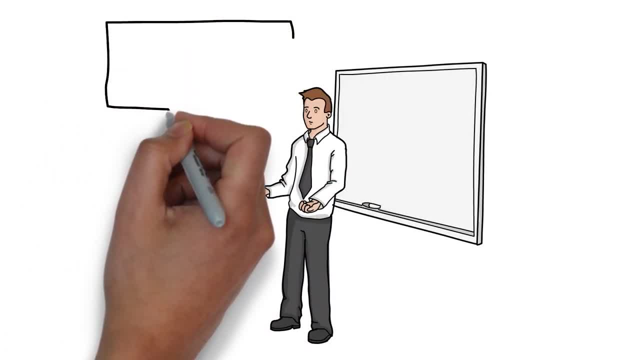 often are not great at conveying information and frequently get lost in detail. And as much as the fine details are important for our work, they may end up shrouding the important concepts that would help the overall process of the trial. In this case, I would like to highlight a few examples. 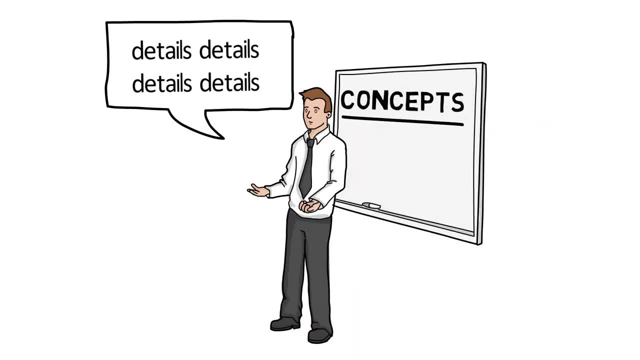 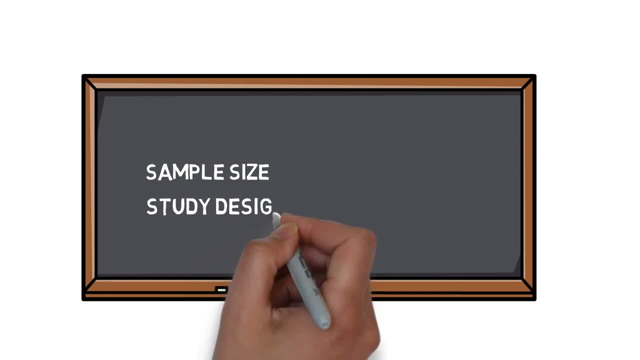 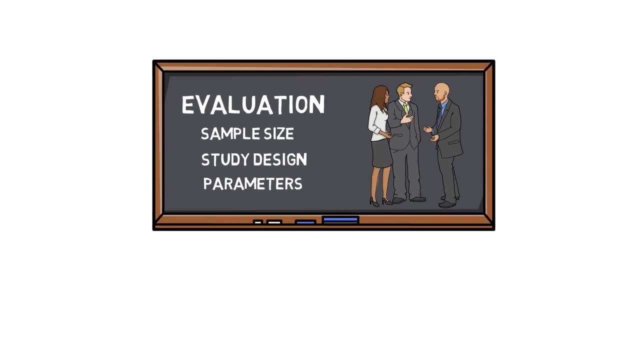 At GCP Service we have made the experience that explaining the bigger picture of what is important for the sample size or the study design and which parameters are important for the evaluation helps the whole study team. This inspired us to look into opportunities to explain these concepts to a wider audience and help inform everyone interested in clinical research. to get a 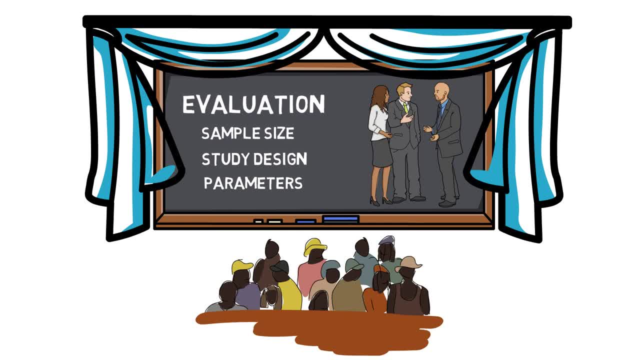 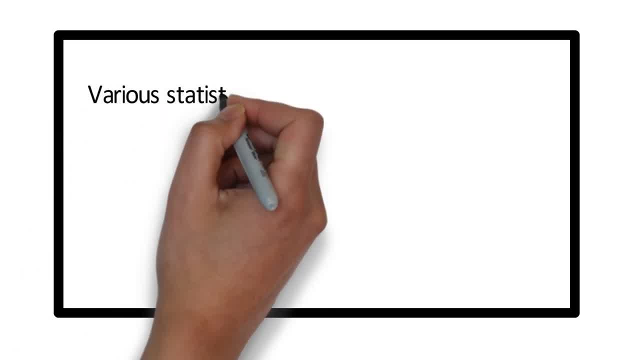 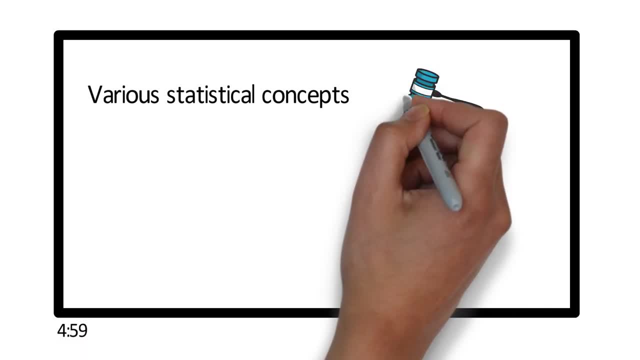 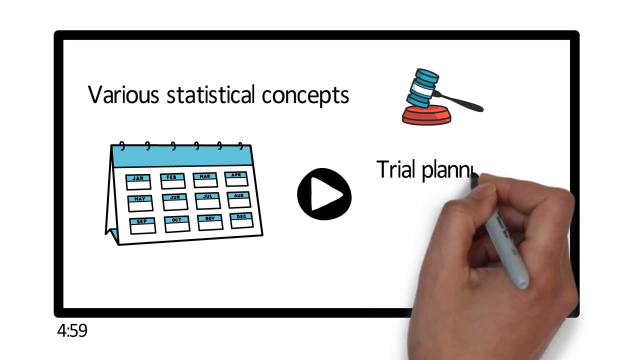 Touching upon various statistical concepts, all presented and visualized in about five minutes to focus on the big picture and help support your decision-making process. Every other week, we will be releasing a video on a new topic, covering information important for trial planning, statistical tests and interpretation of different types of trials.